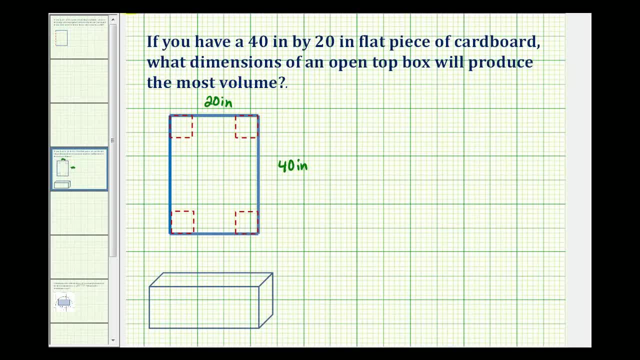 The idea here is: you want to cut out squares from the corner and then fold the sides up to form a box that looks something like this. The issue here is we don't know what size squares to cut out of the corners to maximize the volume. 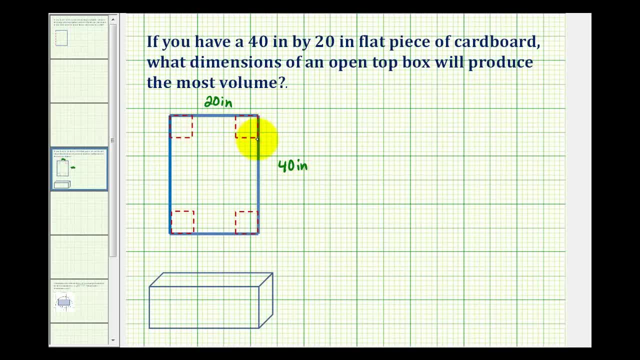 But we do know there are squares, so let's let the length of each side of the square equal x, And all the squares are congruent. So the length of this side, from here to here, would represent this edge on our box, And the length of this side here would represent 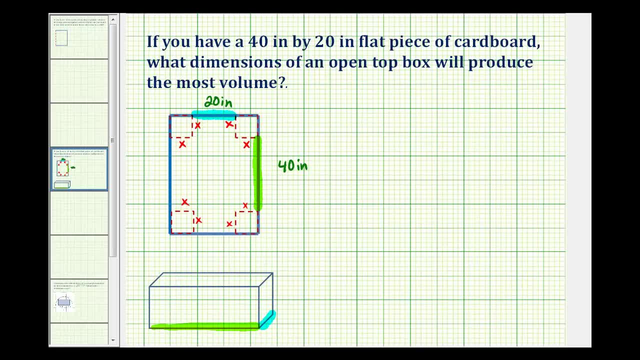 the length of this edge here on the box, And because we're cutting out squares that are x by x, the length of this x here would be the height of the box. So let's go ahead and call this x. Now, if the entire length from here to here 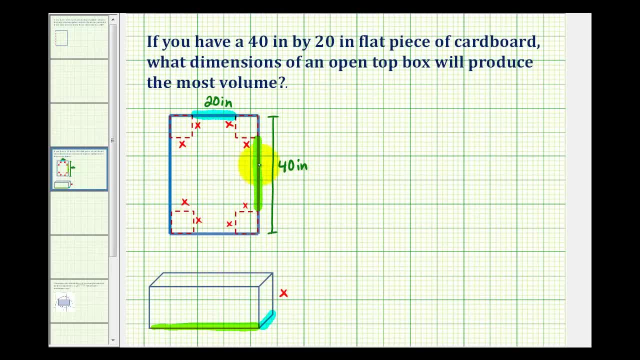 is forty inches, and we take away this length, which is x, and take away this length which is x, forty minus two x would be the length of this green side here. And the same thing happens on this side, If the length from here to here is twenty, and we need the length of this, 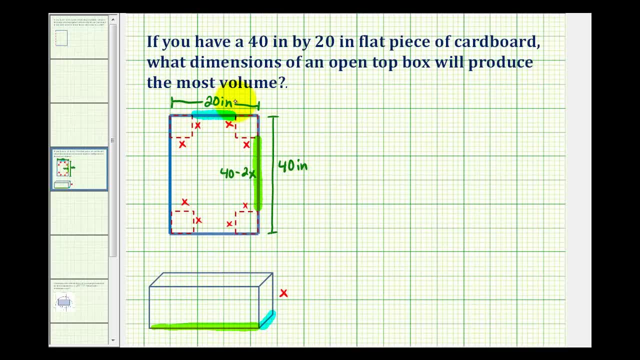 blue segment. here it would be twenty minus x minus x or twenty minus two x. So this edge here would have a length of forty minus two x, And this edge here would have a length of twenty minus two x. So this is all the information we need in order to write. 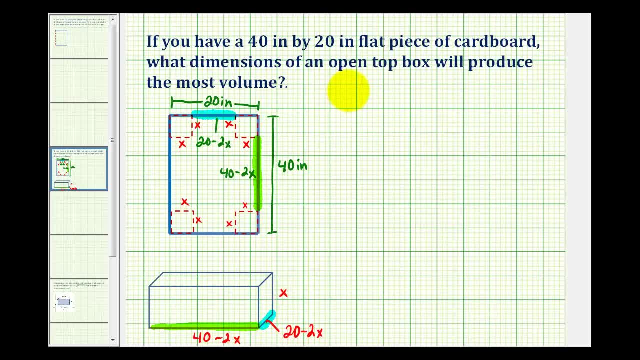 our volume function, The volume of this box is going to be equal to the length times the width times the height, or the product of these three dimensions. So we'll have x times twenty minus two, x times the quantity, forty minus two x. 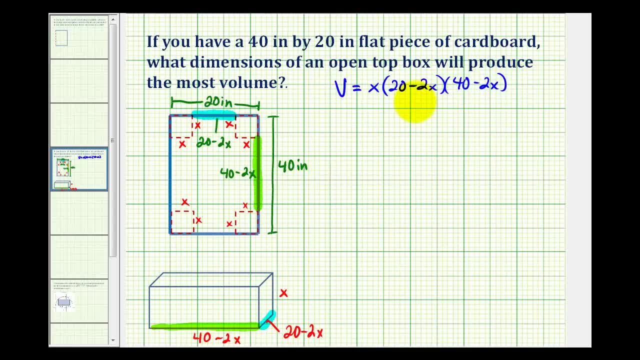 So now we'll determine this product and then maximize our function by determining whether the first derivative is equal to zero. Let's first multiply these two binomials: We'll have eight hundred minus forty x minus eighty x, that's minus one hundred twenty x. 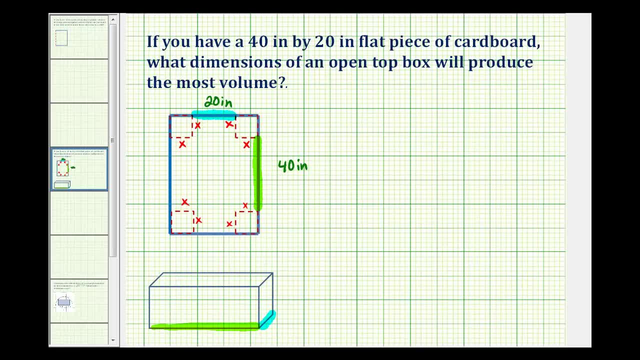 the length of this edge here on the box, And because we're cutting out squares that are x by x, the length of this x here would be the height of the box. So let's go ahead and call this x. Now, if the entire length from here to here 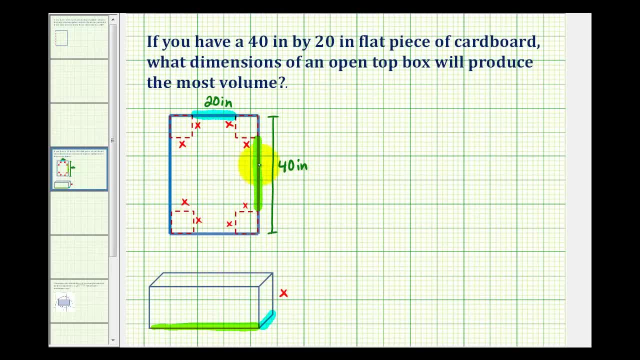 is forty inches, and we take away this length, which is x, and take away this length which is x, forty minus two x would be the length of this green side here. And the same thing happens on this side, If the length from here to here is twenty, and we need the length of this, 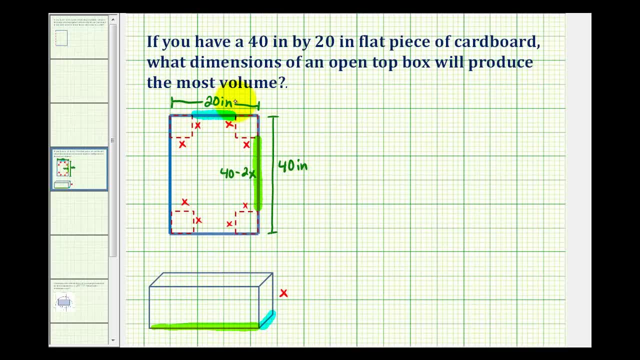 blue segment. here it would be twenty minus x minus x or twenty minus two x. So this edge here would have a length of forty minus two x, And this edge here would have a length of twenty minus two x. So this is all the information we need in order to write. 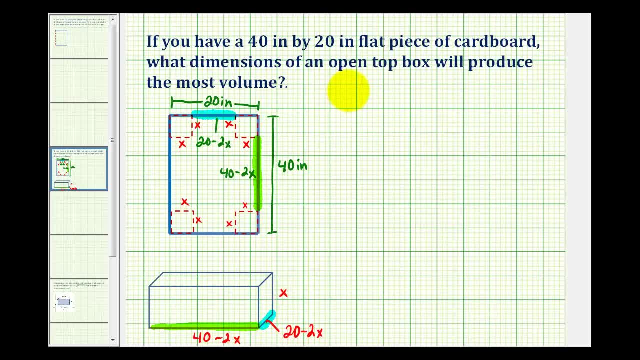 our volume function, The volume of this box is going to be equal to the length times the width times the height, or the product of these three dimensions. So we'll have x times twenty minus two, x times the quantity, forty minus two x. 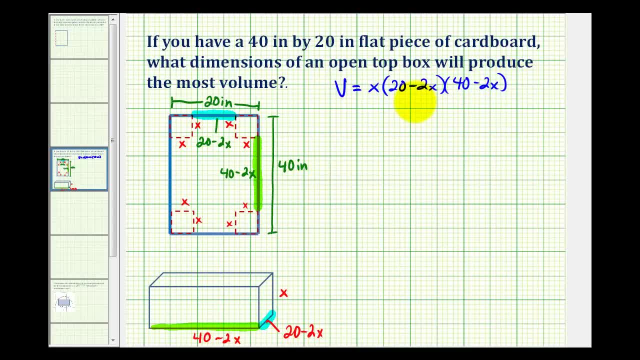 So now we'll determine this product and then maximize our function by determining whether the first derivative is equal to zero. Let's first multiply these two binomials: We'll have eight hundred minus forty x minus eighty x, that's minus one hundred twenty x. 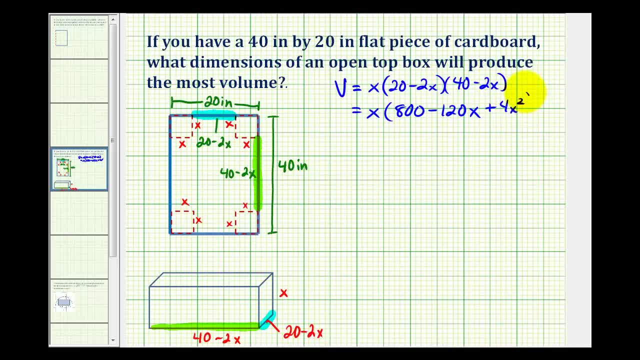 and then plus four x squared. Now we'll distribute the x, and I'm going to go ahead and put these terms in descending order. So I'll have four x cubed minus one hundred twenty x squared, plus eight hundred x. So now to determine the maximum volume. 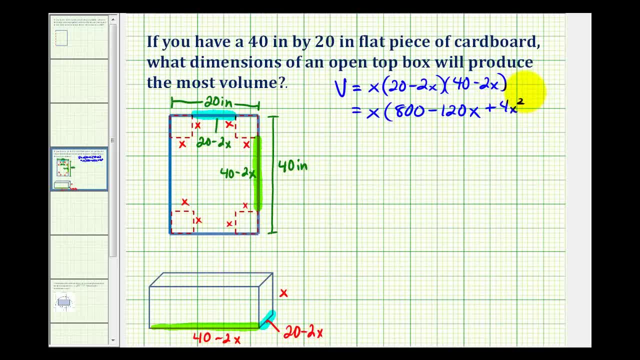 and then plus four x squared. Now we'll distribute the x, and I'm going to go ahead and put these terms in descending order. So I'll have four x cubed minus one hundred twenty x squared, plus eight hundred x. So now to determine the maximum volume. 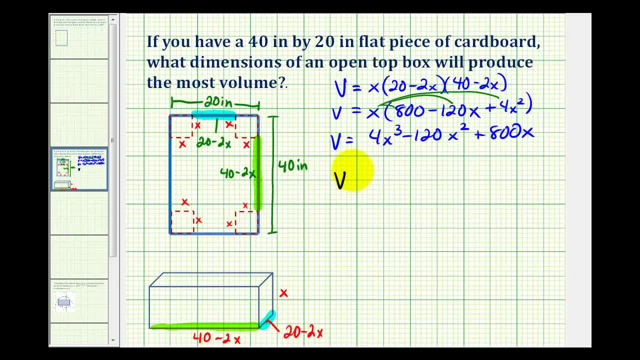 we'll find the derivative and determine whether the derivative is equal to zero or does not exist. So we'll have twelve x squared minus two hundred forty x plus eight hundred. Now the derivative is a polynomial function, So it will exist for all values of x. So let's go ahead and set this equal to zero and solve. 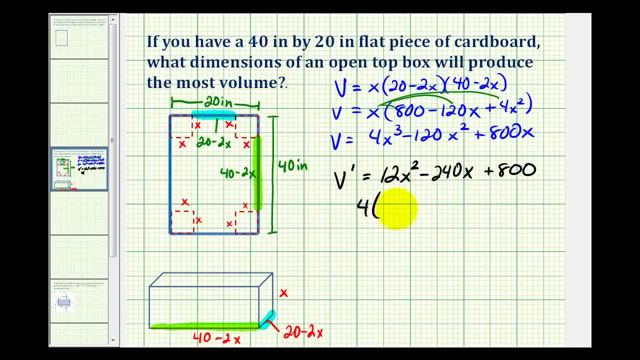 We can factor out a four from these three terms, So we'll have four times the quantity. three x squared minus sixty x plus two hundred equals zero. Now, unfortunately this does not factor, So that means we have to determine the critical numbers. 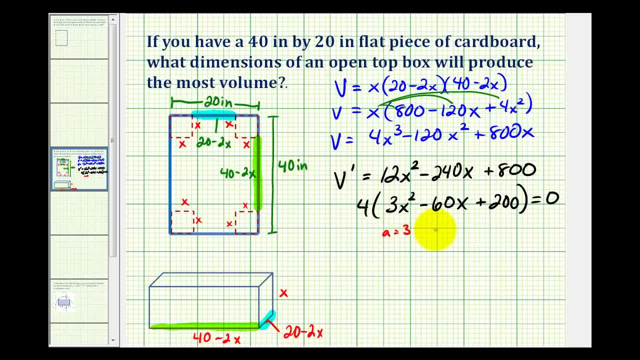 by using the quadratic formula. So we'd have a equal to three, b equal to negative sixty and c equal to two hundred, And the quadratic formula is: x equals negative, b plus or minus the square root of b squared minus four, a, c all over two a. And to save some time, I've already done this. 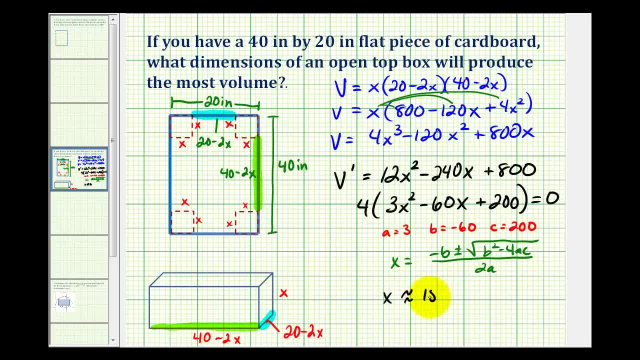 The solutions would be: x is approximately fifteen point eight and x is approximately four point two. But notice how we still don't know if these x values produce maximums or minimums for the volume. But there is one thing that we can do. 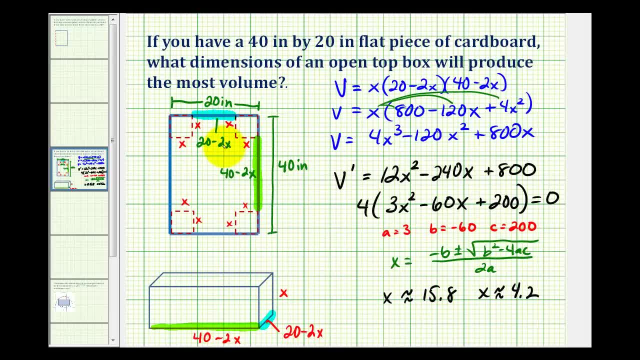 Notice how the length of this side here is twenty minus two x. So if x was equal to fifteen point eight, the length of this side here would be negative, which obviously is not possible. So we can exclude this as a possible value of x, But we do want to verify that this. 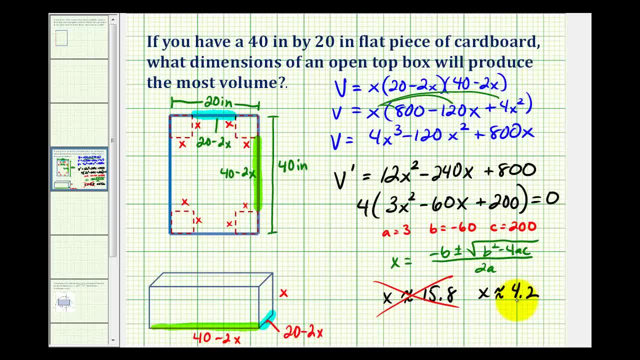 x value does produce a maximum, And we can do that by determining if the function is concave up or concave down at this value of x. So we'll determine the second derivative of the volume function and then evaluate it at x equals four. point two: 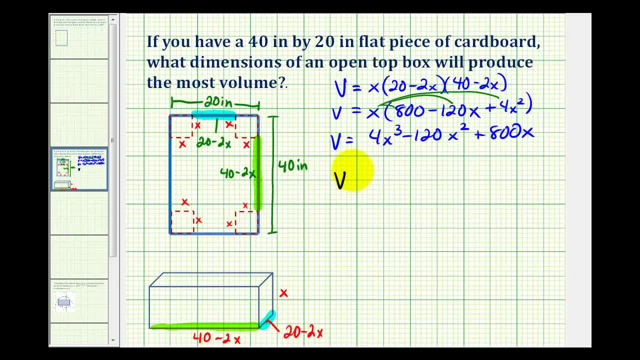 we'll find the derivative and determine whether the derivative is equal to zero or does not exist. So we'll have twelve x squared minus two hundred forty x plus eight hundred. Now the derivative is a polynomial function, So it will exist for all values of x. So let's go ahead and set this equal to zero and solve. 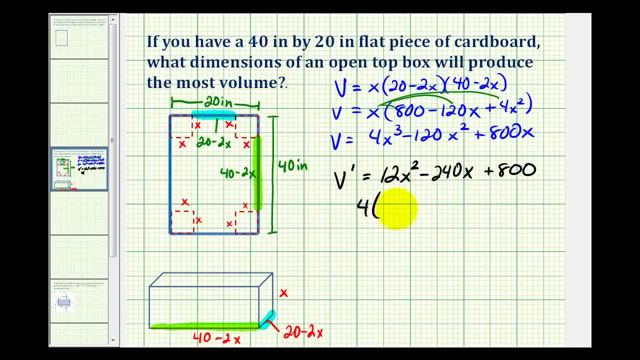 We can factor out a four from these three terms, So we'll have four times the quantity. three x squared minus sixty x plus two hundred equals zero. Now, unfortunately this does not factor, So that means we have to determine the critical numbers. 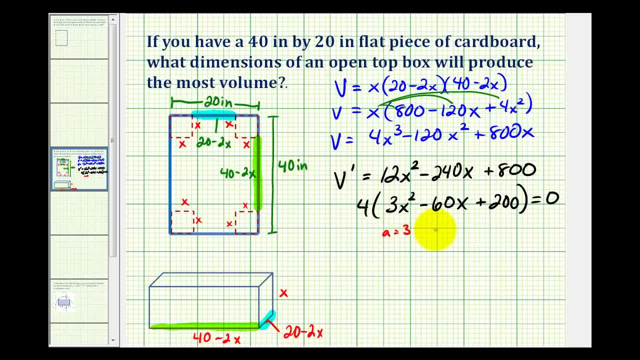 by using the quadratic formula. So we'd have a equal to three, b equal to negative sixty and c equal to two hundred, And the quadratic formula is: x equals negative, b plus or minus the square root of b squared minus four, a, c all over two a. And to save some time, I've already done this. 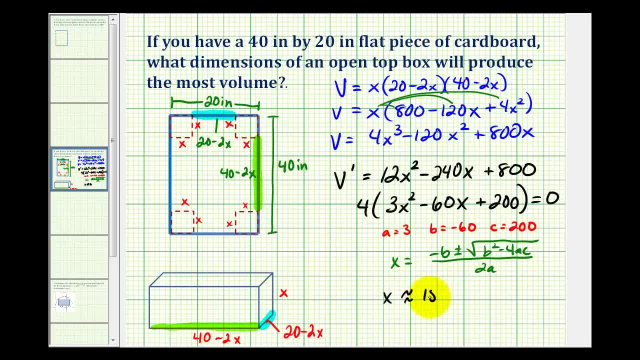 The solutions would be: x is approximately fifteen point eight and x is approximately four point two. But notice how we still don't know if these x values produce maximums or minimums for the volume. But there is one thing that we can do. 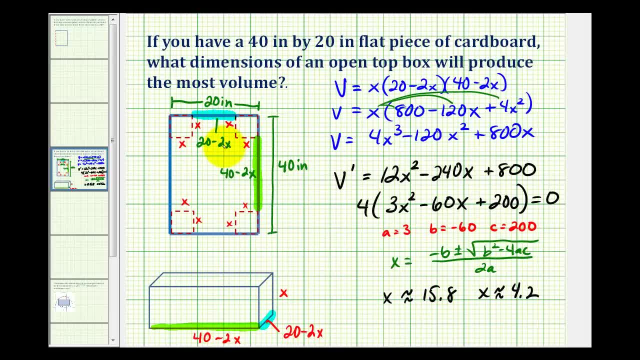 Notice how the length of this side here is twenty minus two x. So if x was equal to fifteen point eight, the length of this side here would be negative, which obviously is not possible. So we can exclude this as a possible value of x, But we do want to verify that this. 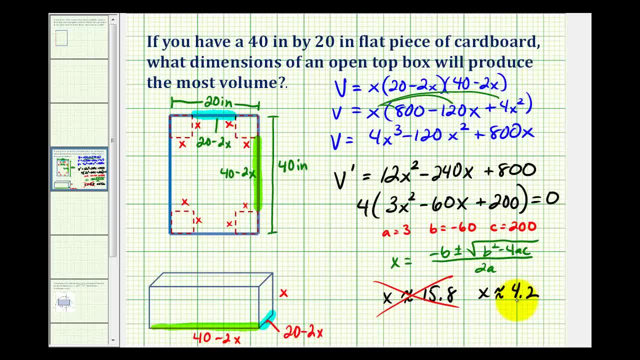 x value does produce a maximum, And we can do that by determining if the function is concave up or concave down at this value of x. So we'll determine the second derivative of the volume function and then evaluate it at x equals four. point two: 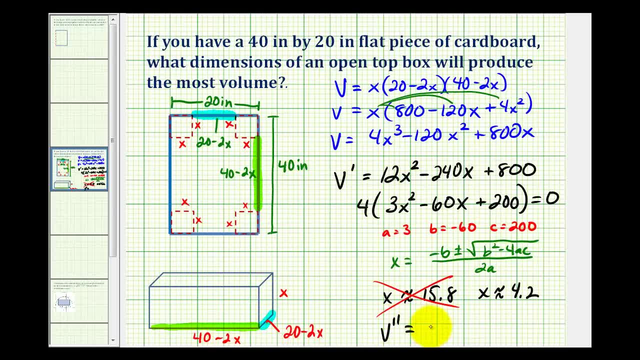 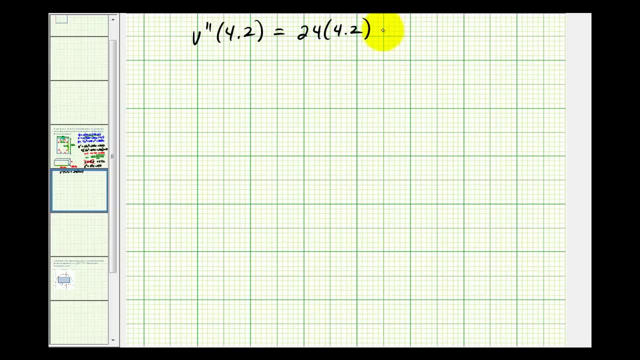 So the second derivative of the volume function would be twenty four x minus two hundred forty. So now let's evaluate this at: x equals four point two. This is going to be one hundred point eight minus two hundred forty, which is obviously going to be.